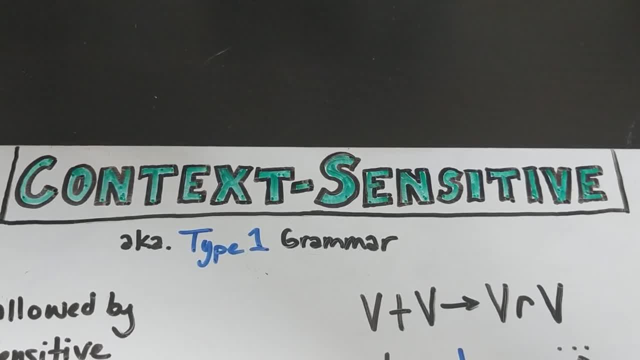 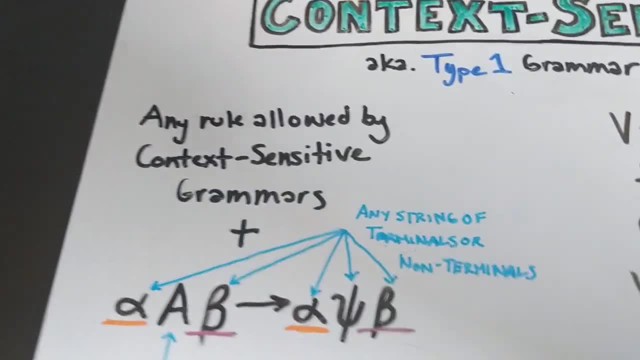 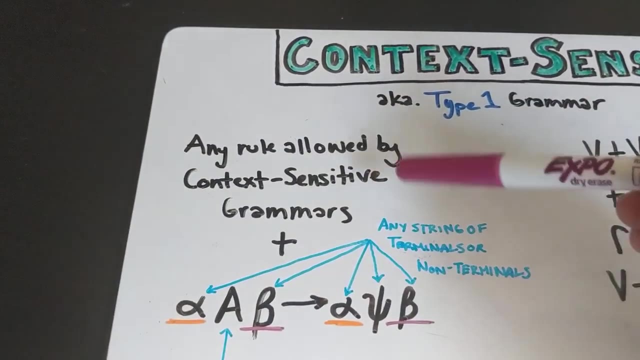 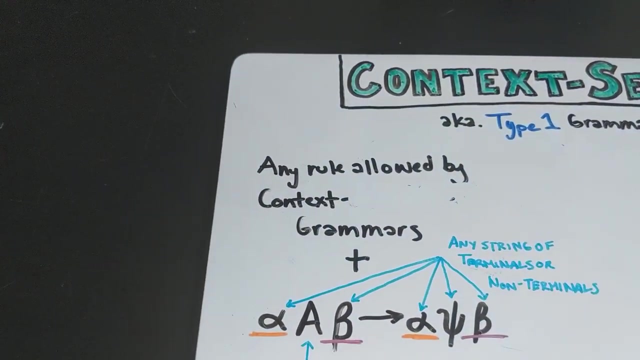 we're doing with that in the last video. This is also called the type 1 grammar, because it's the most complex of the slightly restricted grammars. So this is how we describe a context-sensitive grammar. So, first of all, any rule that's allowed by a context-free grammar is allowed. 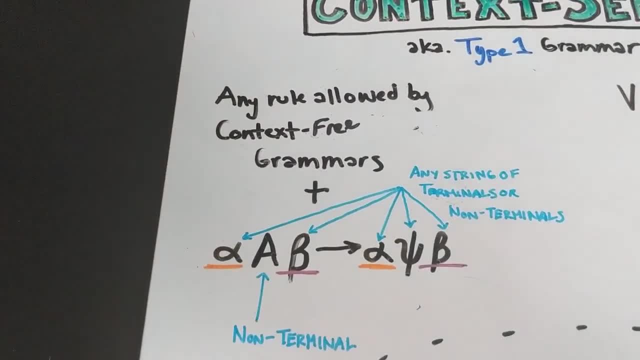 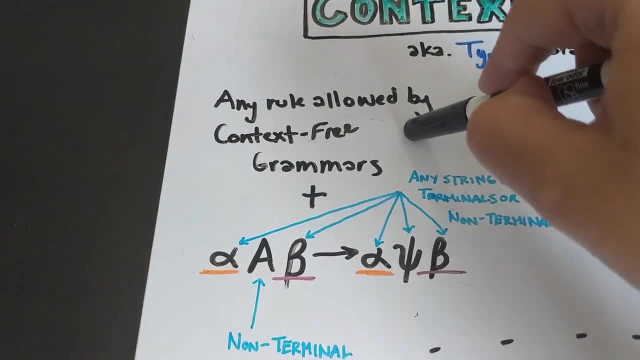 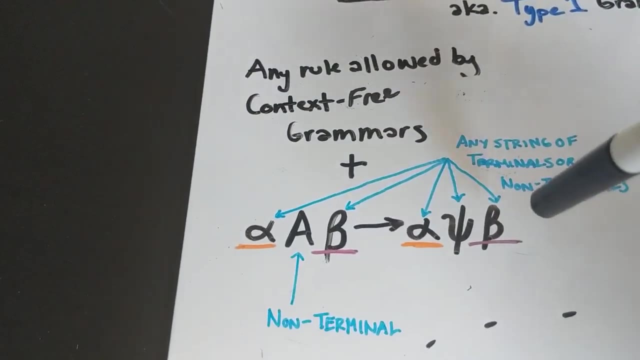 by a context-sensitive grammar, Which also means, because any rule that's allowed by a regular grammar is allowed by a context-free grammar, you can also have any rule that's allowed by a regular grammar. Alright, so any of the rules we've talked about before, plus any rule that has this. 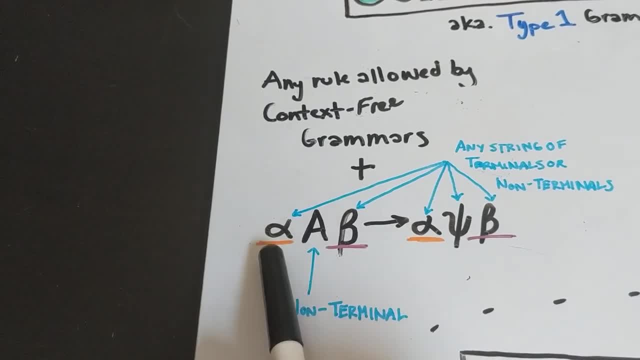 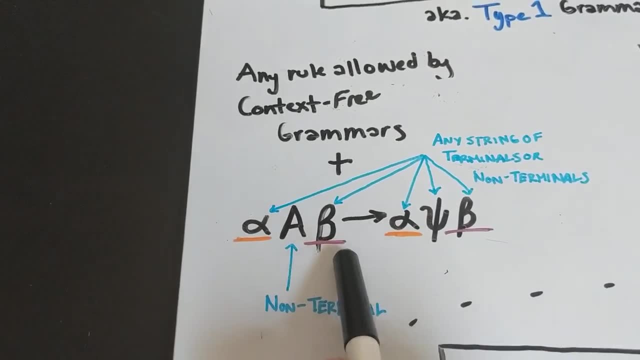 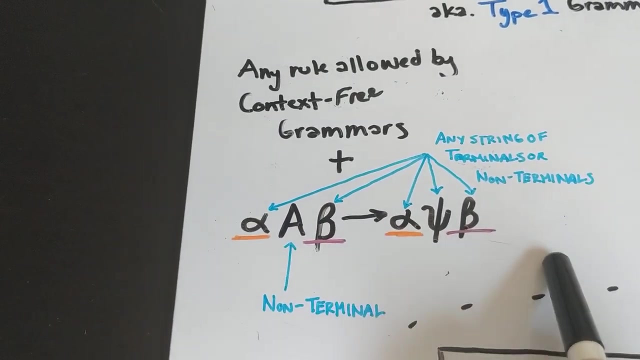 format. So what this says is that we have some string of terminals and non-terminals followed by a non-terminal, followed by some string of terminals and non-terminals, followed by is equivalent to, is equivalent to some string of terminals and non-terminals where these two strings 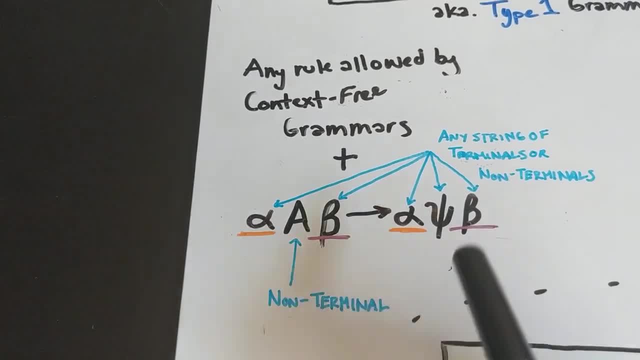 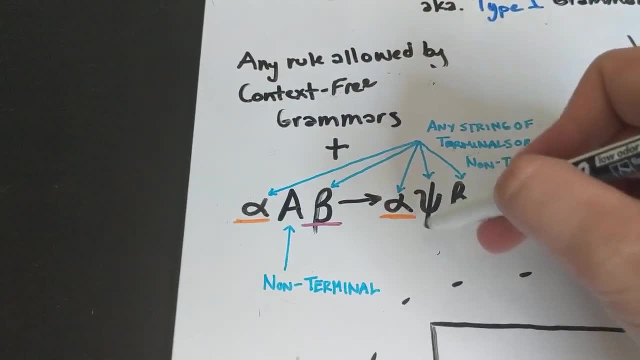 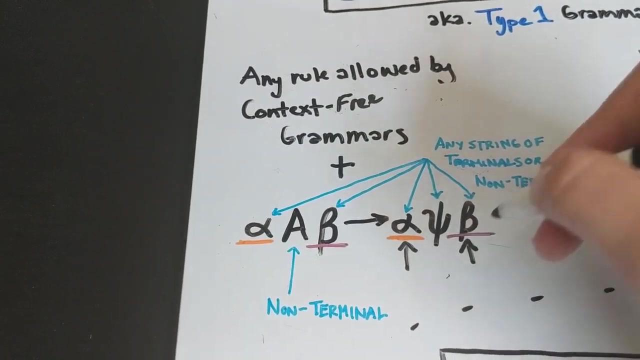 have to be the same, and these two strings have to be the same. So what does that mean? That means, basically, that this a can be replaced by any string of terminals and non-terminals, so long as it's bracketed by the same stuff. Right, As long as it remains bracketed by. 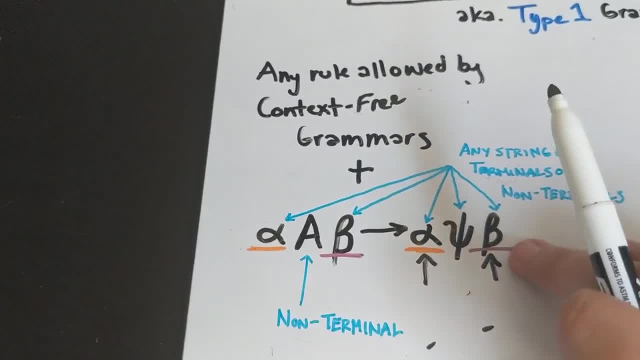 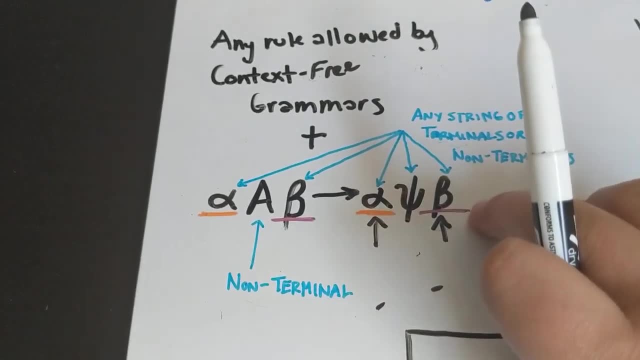 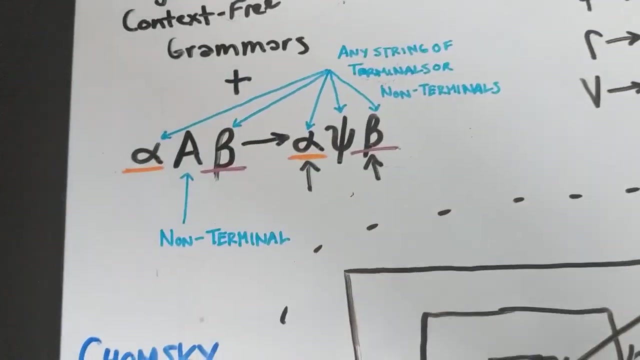 the same stuff. Now, this is not. This is still more restricted than the definition of how you make grammar rules. So we'll talk about this in a second, about why we're still restricting it, even though it's the most complicated of the grammars that we're going to talk about. 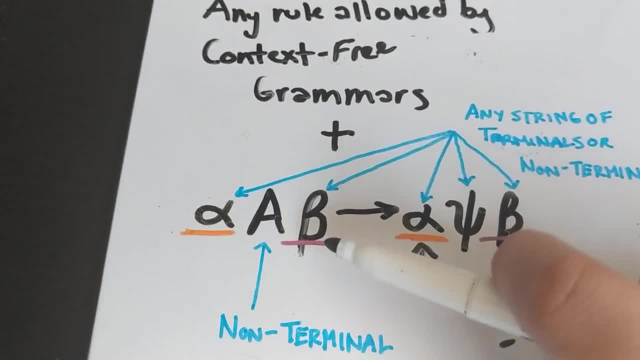 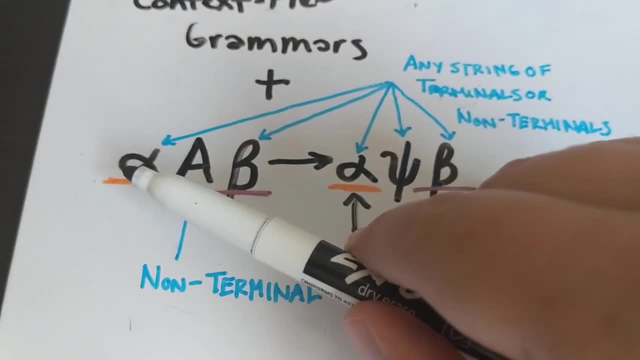 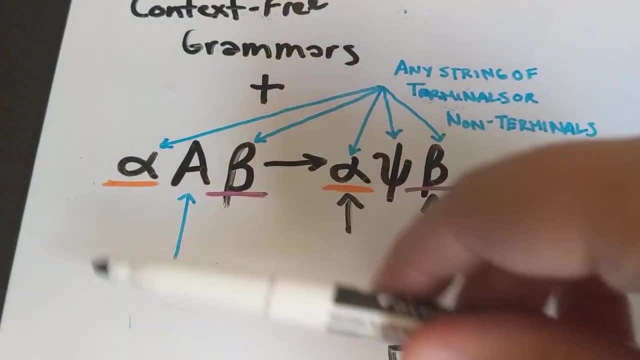 So essentially what this means is you can have any string of terminals and non-terminals so long as you have a non-terminal in there, But that whatever you've got on the left has to be preserved and whatever you've got on right has to be preserved, and then you can fill in whatever you want in between. 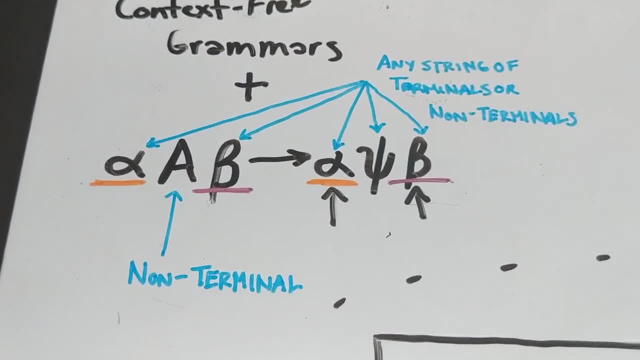 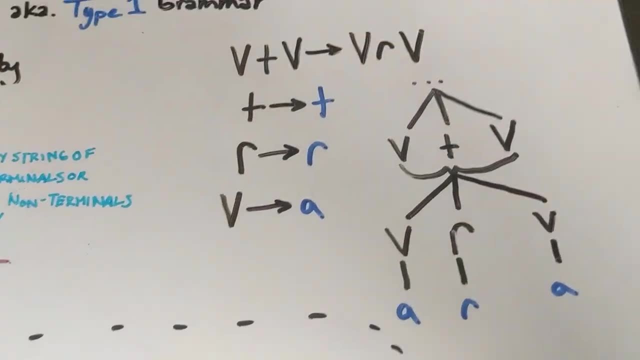 So that's basically what this requires. So if we go back to the example that we touched on last time, that we couldn't account for using a context-free grammar, let's look at that. So we've created some rules here where we have a non-terminal V followed by a non-terminal 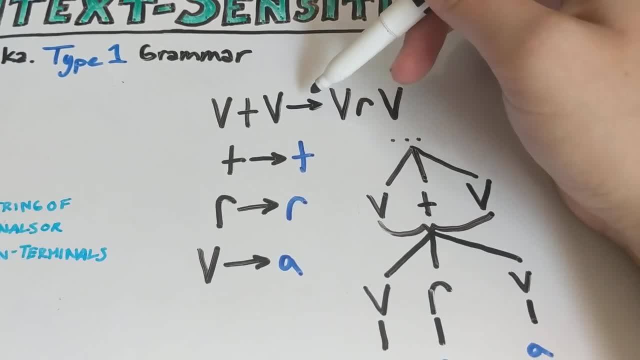 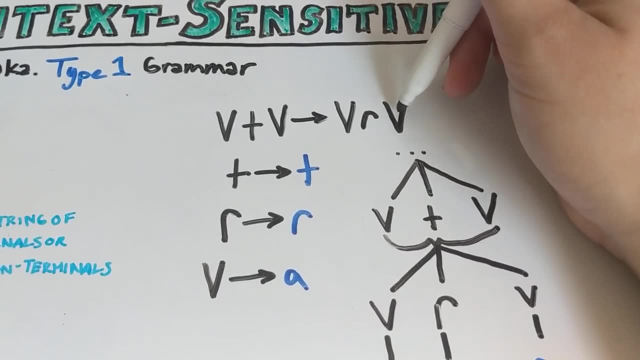 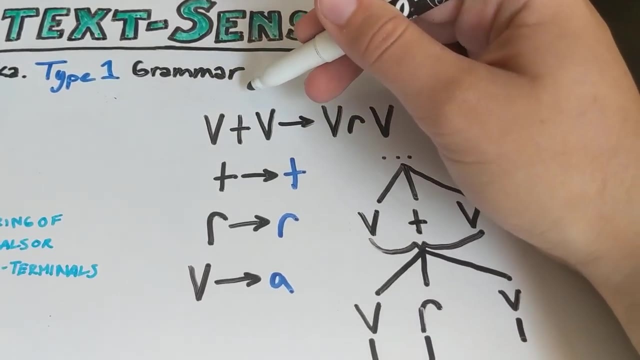 T followed by a non-terminal V is made up of a non-terminal V followed by a non-terminal flap, followed by a non-terminal V, right. This is a rule that you cannot do in context-free grammars, because we've got more than one non-terminal. 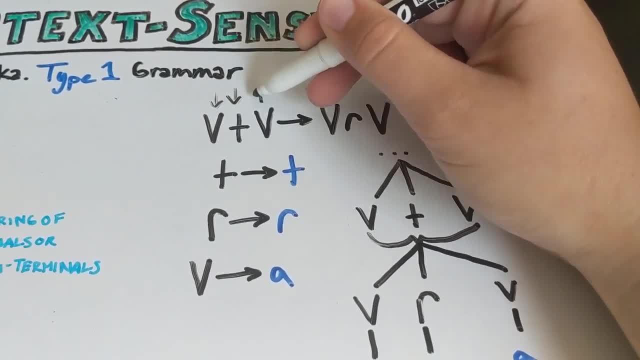 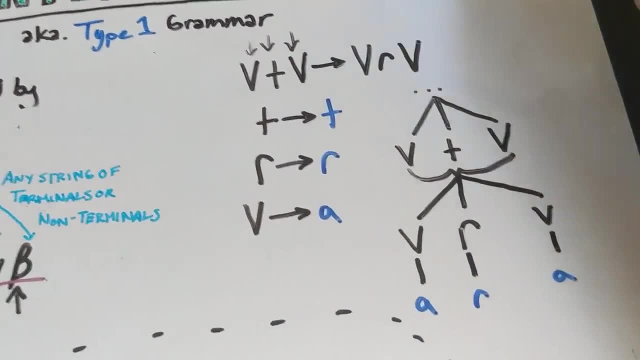 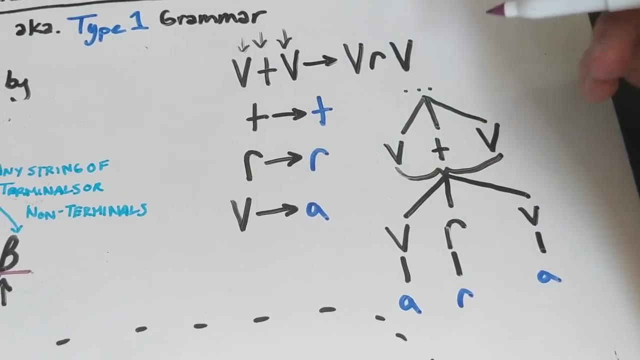 on this side. right, we've got three, And so a context-free grammar would not like that rule. The rest of these rules would be fine in even a a regular language. so the rest of these rules just tell you how we break this down. 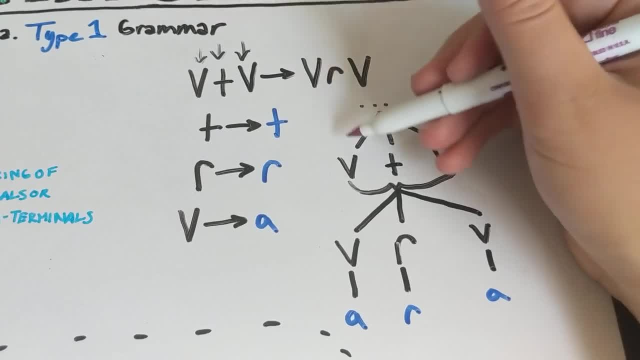 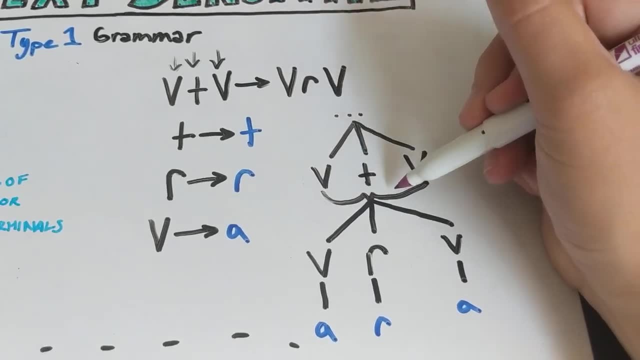 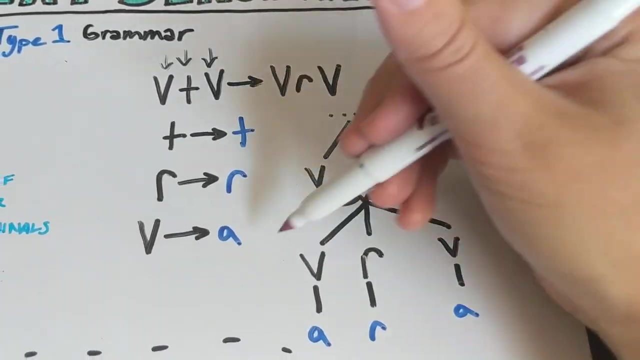 So imagine that you know whatever has you know been above here in our structure, we have this sequence. We're going to take this whole sequence right, so this no longer works very well in a tree, right? we're going to take this whole sequence and replace it with this whole sequence, right? 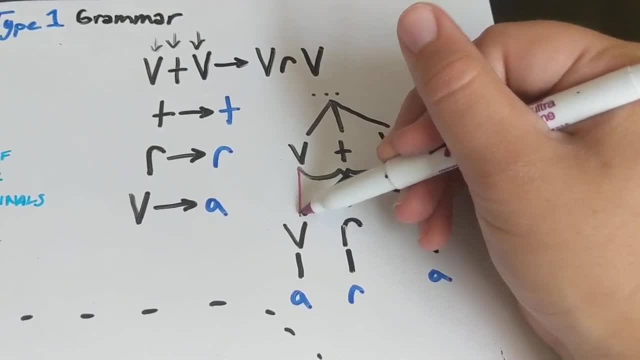 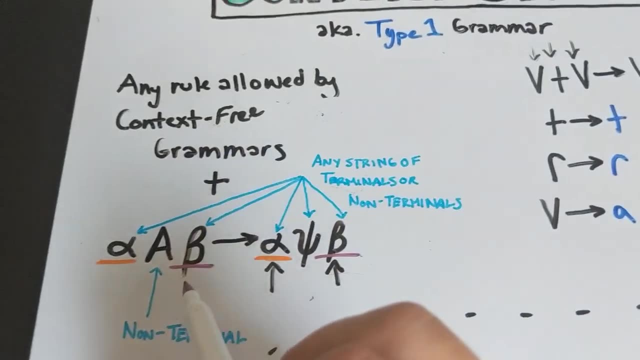 So we still have a V and a V on the side right, so we could maybe draw lines. Do you see that Down there right We still have the V and the V on the sides, which is alpha would be V and beta would be. 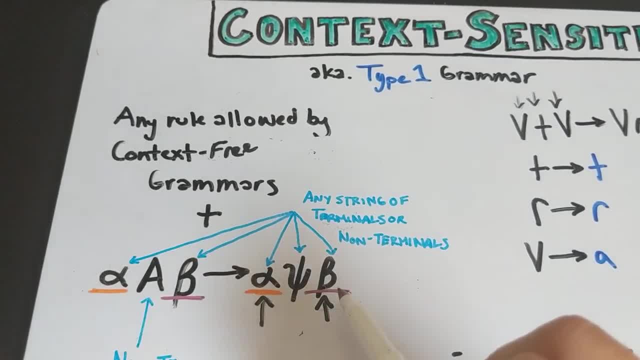 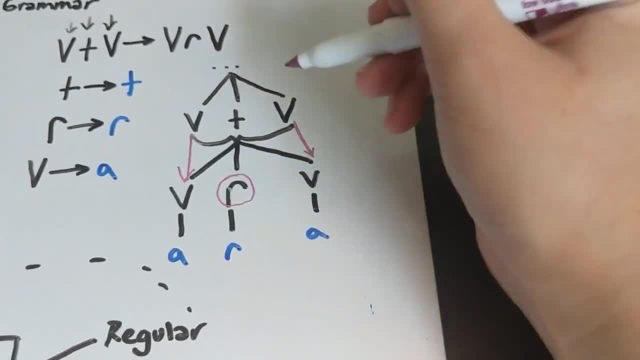 V, right, So we still have the V and the V on the sides, but the resulting sequence is a little bit different because we've got a different non-terminal in here, right, And then from there we can just apply our rules, and so this is this: lets us have. 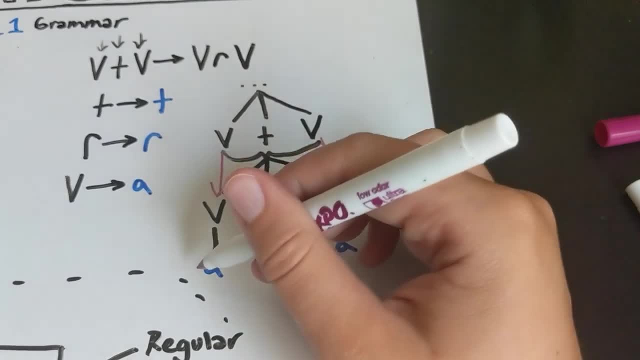 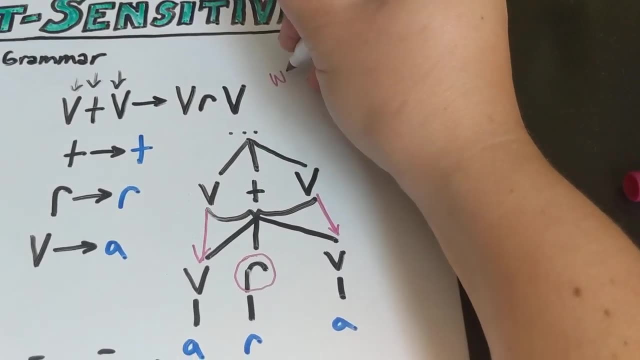 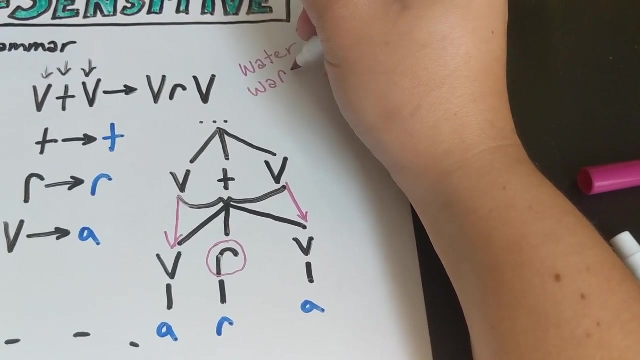 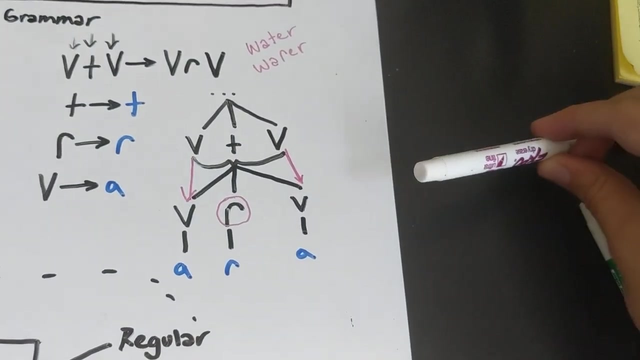 ata instead of ata, which we don't see in in standard American English right, We say water. We don't say water. we say water. And if you're not understanding this, make sure you watch the previous video, because I explained this whole thing in the previous video. 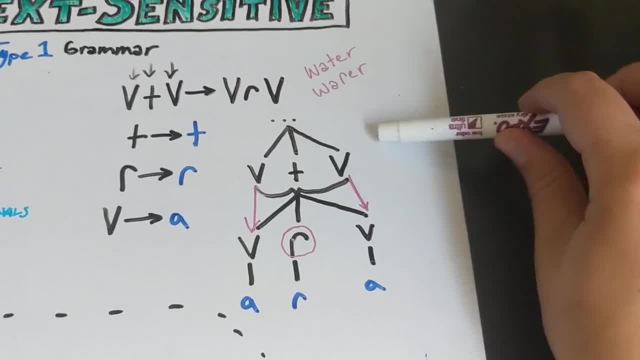 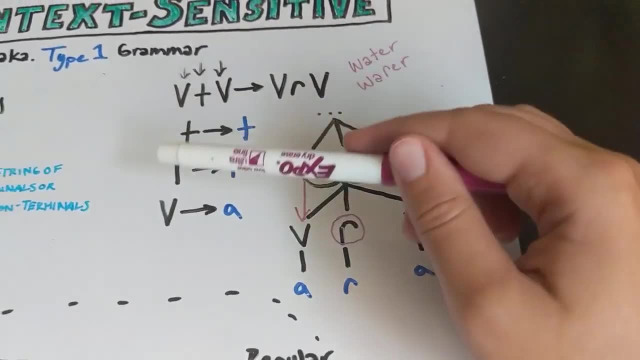 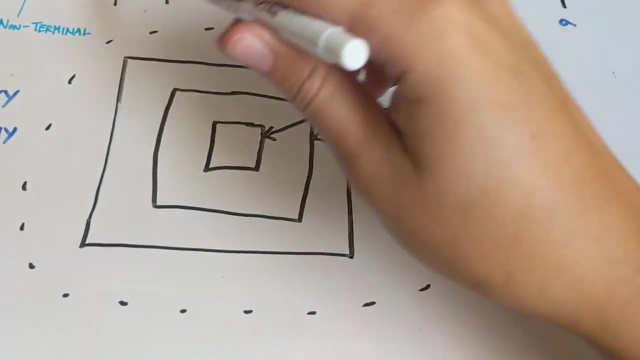 So this is a context-sensitive language. It's a lot harder to represent in a tree like this, but it places fewer restrictions on the types of rules You can make. So what do we have altogether? What we have is sort of a series of embedded different types of grammars, right?